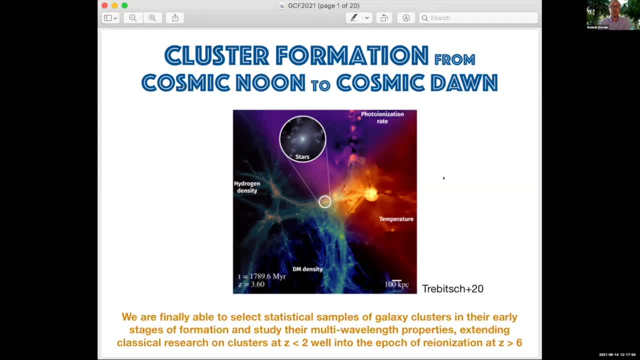 Maybe not completely, Not quite at the level of detail as provided by these wonderful hydro simulations of forming clusters, as in this example I show here, but maybe at the sufficient level of detail that we can start comparing data with with theory and constrain the theory. 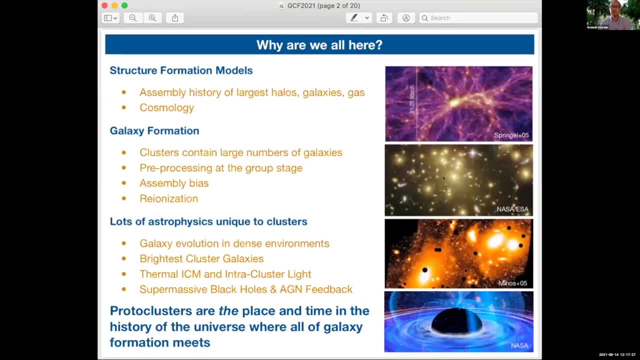 So let me also try to summarize why I think we are all here. The story of cluster formation is the story of the history Of the largest objects in the universe, And this is, of course, closely related to the cosmology From a general galaxy formation standpoint. 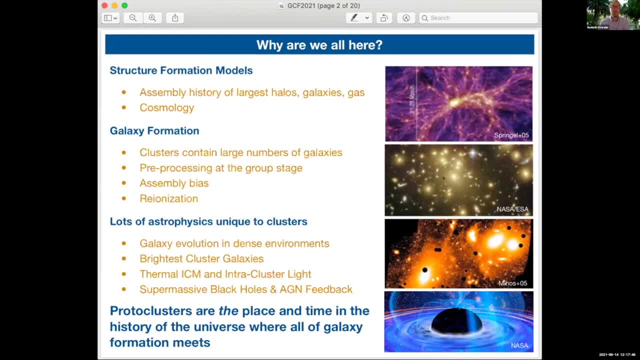 I think we're really missing important pieces of the puzzle if we only only focus on field galaxies. clusters contain large numbers of go evil galaxies that may have affected each other and their surroundings on length scales and time scales That are much larger than those for typical galaxies. 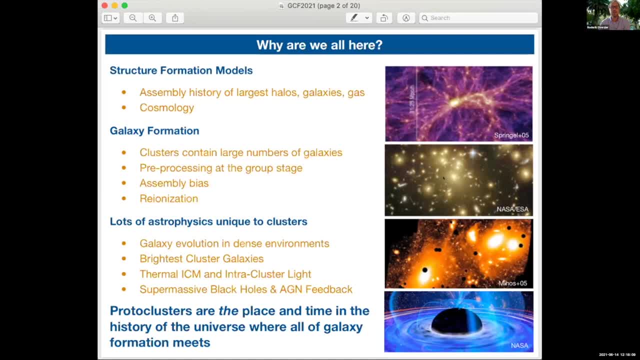 And even if the physics that is happening in galaxies in clusters and project clusters may not be different than the physics that affects galaxy formation in general, There is at least a lot of unique astrophysics that is exclusively found in clusters and their progenitors. 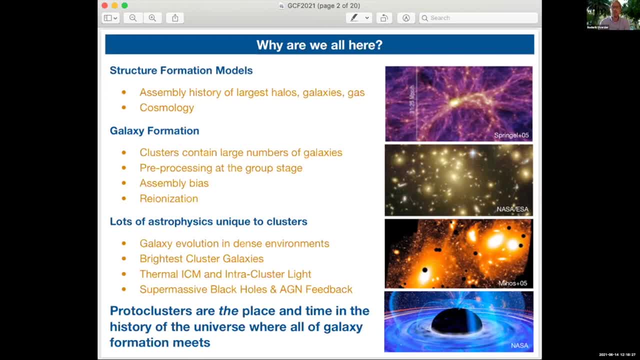 And then I'm thinking of galaxy evolution in dense environments, Brightest cluster galaxies, The inter cluster medium and the inter cluster night lights, And also unique forms of AGM feedback and super massive, super massive black holes. So I think this field is incredibly rich and I like- I like to see proto clusters as as the time and place in history of the universe where all known aspects of galaxy formation are happening, as no doubt we will see during this week. 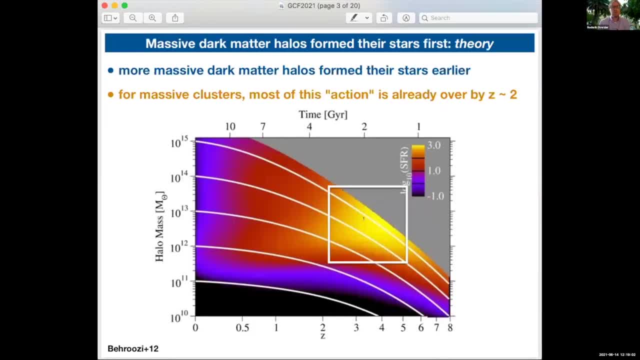 Thank you. From a theoretical perspective, we've known for for quite some time that the more massive the dark matter halo, the earlier it formed in stars on average. This is a nice figure from the work of the Lucy at all that I like to show. it shows you the mass evolution of dark matter halos. 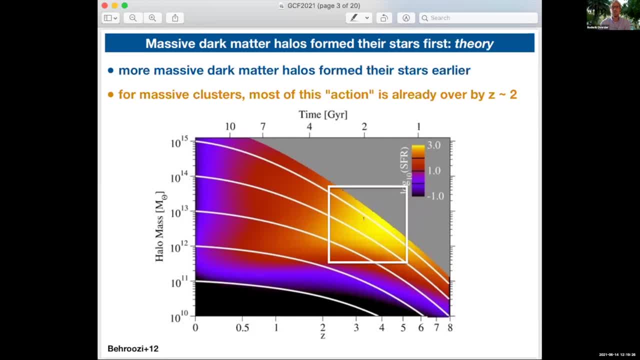 And this is color coded by their star formation rates. So if you now focus on the progenitors of Of the most massive halos, Then you see that their star formation really peaks at very high redshifts above certainly about Richard too, And so that means that for for massive clusters, most of the action happens at at very high redshifts. 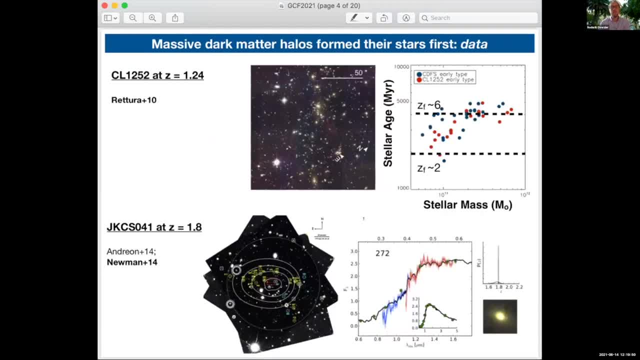 And we also noticed from an observational perspective based on galaxy clusters. The two examples I show here are probably not representative. They are rather extreme clusters at their respective redshifts of 1.2 and 1.8.. The example by that to a little too intense shows you the derived stellar ages of the cluster ellipticals in the co 1252 as function of their stellar mass. 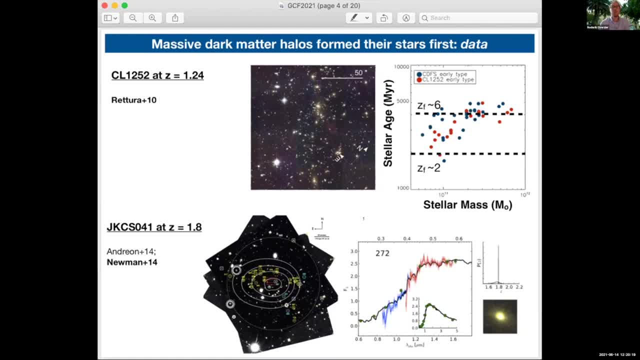 And so for most of these cluster ellipticals, their stellar populations have ages very close to ratchet of 456.. And at the bottom, The cluster about to 1.8- study by on the own at all Newman at all, which is a remarkable- objects with the quiescent fraction of 80%, something like this. 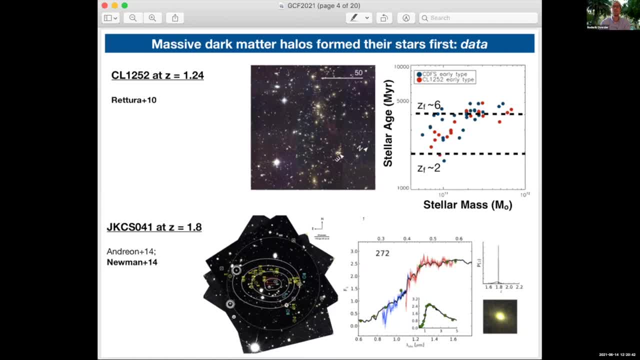 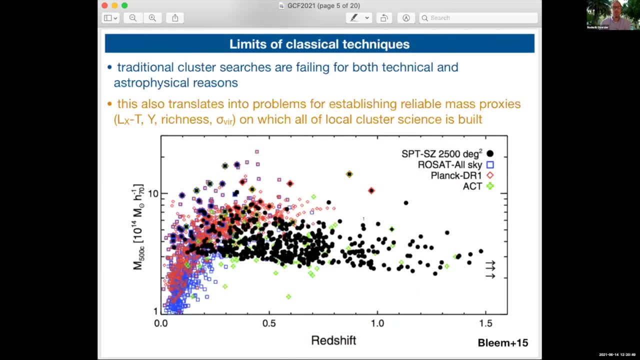 And so for these systems, we have missed all of the all of the action that led to the formation of the system. I think we all know that the classical cluster search techniques have Have been have limitations. these limitations limit our samples and selections to redshift 1.5 to 2 or so. 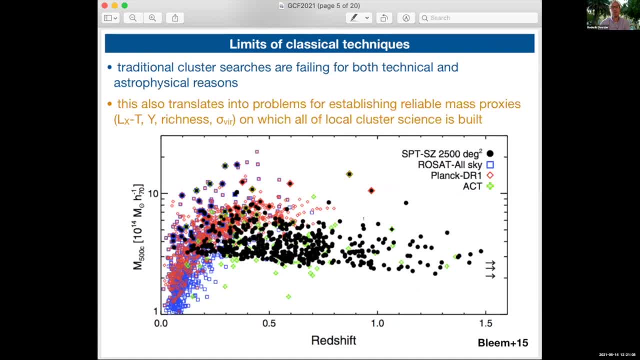 these traditional searches are failing not only for technical reasons- right x-ray sensitivities, etc. but also for astrophysical reasons. so the, the components of clusters that we are used to look for, simply did not exist yet before these clusters became clusters. but it also translates into problems for establishing reliable mass proxies, on which all of local cluster science 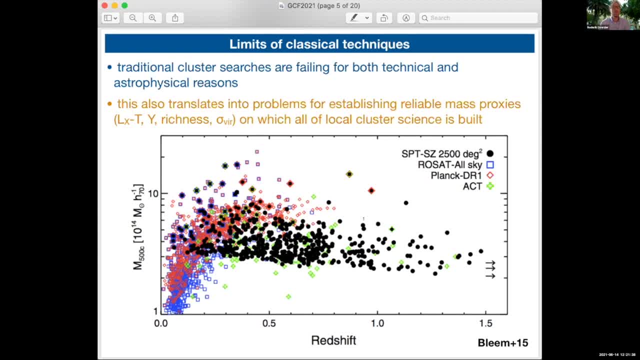 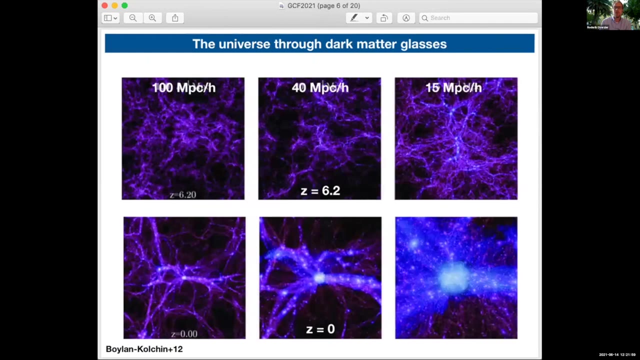 is built. so think of the luminosity temperature relation, the compton y parameter, the richness class or the velocity dispersion to get a virial mass. so most of this is becomes pretty no disrespect, useless above redshift about freshness too. now if we were to put on our 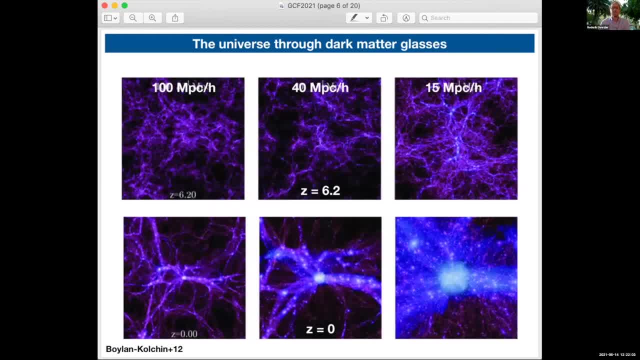 dark matter glasses for a minute. then if we look up the sky, i think we would have no problem whatsoever to just find out where all the interesting structures are forming. and we can do this to very high redshifts, as you see here in this millennium xxl simulation at redshift 6. 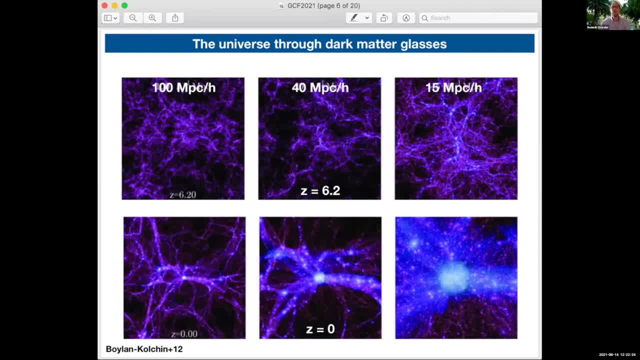 depending on the scale you're looking at, it will be very easy to point out where the progenitors of massive clusters are are assembling. now, unfortunately, we don't have such glasses, but mixed in with the dark matter, there will be gas and galaxies that we can detect, and so it really becomes a question. 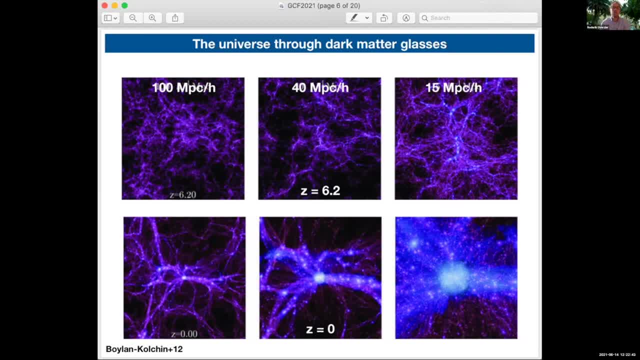 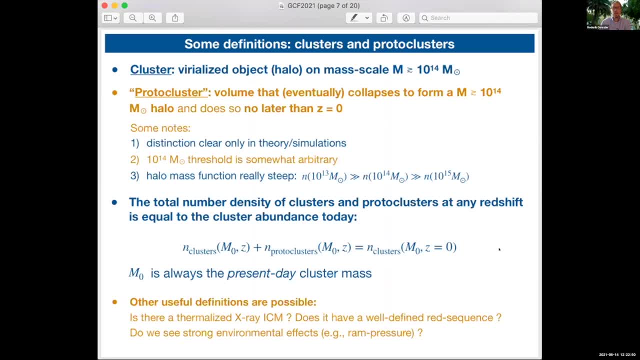 of what should we be searching for and whether our telescopes are are big enough to to to detect these systems. i think it's important to talk about some basic definitions. none of these definitions are hills that i'm willing to die on, but i think we should make an attempt to to agree on what, what we're. 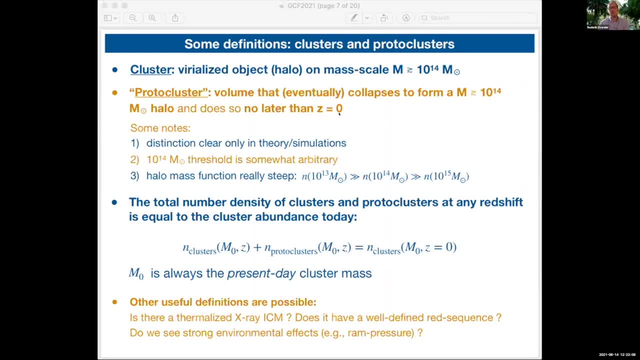 talking about. so in in this, this, this talk. when i say cluster, i'm thinking of virilized objects, single dark matter, halos on a mass scale of at least 10 to the 14 solar masses, and then that's thezięki taking his thing of worries. vraivox' frame receive some sevenths of a man like that. 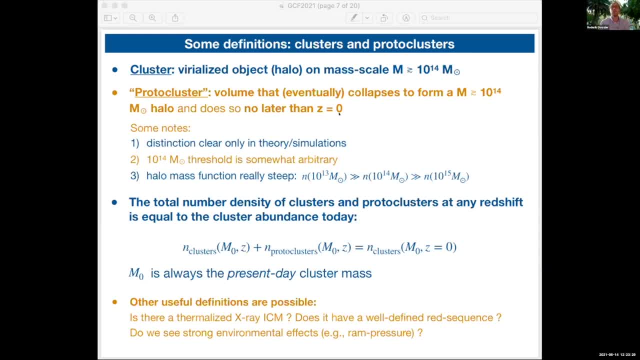 make sense so you can create. i think this was a profound numa. just i tried like this before sum it up. so um oh, 14 solar mass threshold is somewhat arbitrary, but i think it makes sense because the halo mass function is really steep at these high masses. so there's uh orders of magnitude more galaxy groups. 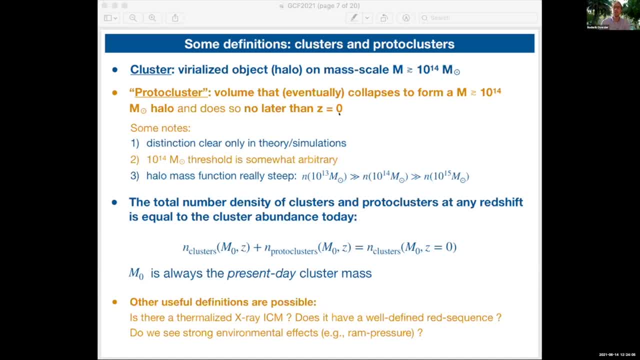 than there is of uh. then there are 10 to the 14 solar mass clusters, and those are orders of magnitude more common than 10 to the 15 solar mass clusters. so some kind of mass distinction is important. an advantage of this definition is that then the total number, density of clusters 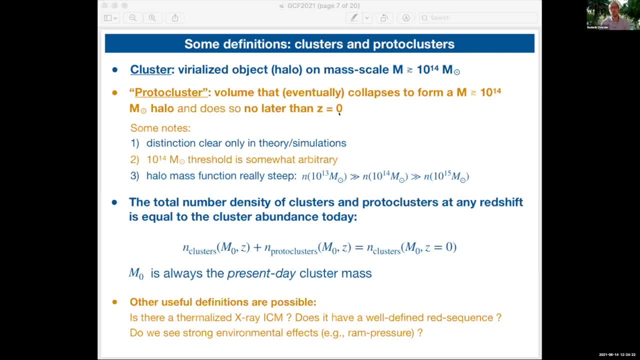 and proto clusters at any redshift will be equal to the cluster abundance today. but i'm well aware that there are other useful definitions possible and also being used by you and, for example, sensible questions to ask are: is there a thermalized x-ray icm or not? does the object have a well-defined threat sequence? 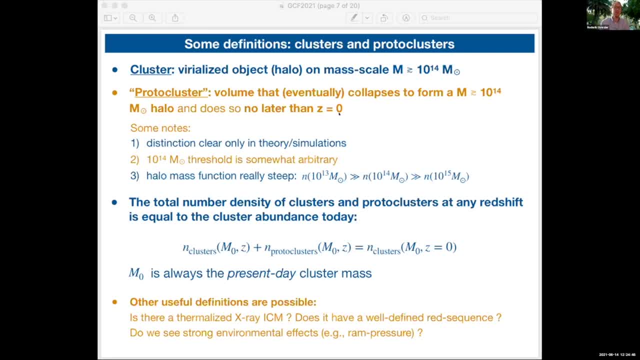 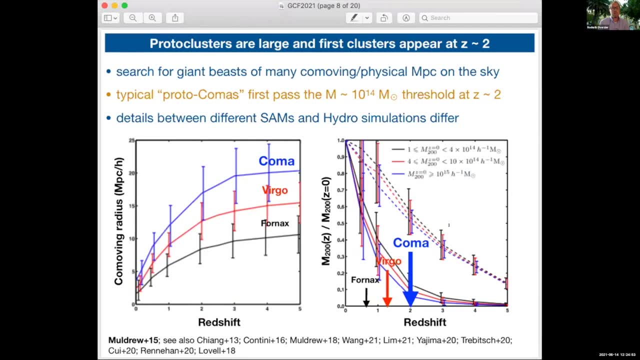 or do we see the beginnings of strong environmental effects like ram, pressure or ground against the current, in future generations? now for um, we have known for quite some time that, at least from from a theoretical perspective, we should have no problem of identifying these kind of structures, uh, before they they've been realized. 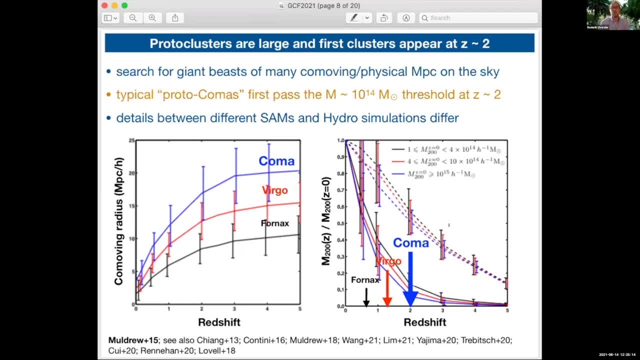 and uh work from semianatic models- uh principally- has shown that we should be looking for giant beasts covering many co-moving physical megaparsecs in the sky. and we've also learned that the typical progenitor of a coma cluster first passes this 10 to the 14 solar mass cluster threshold at a. 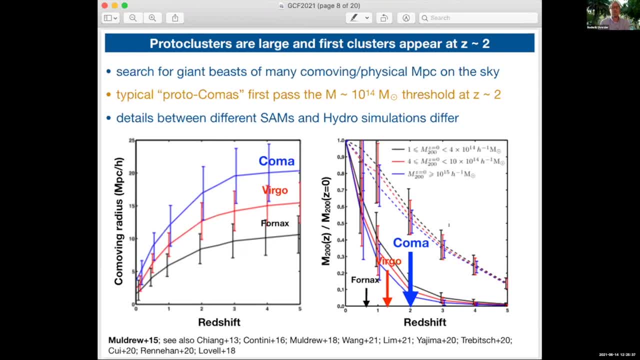 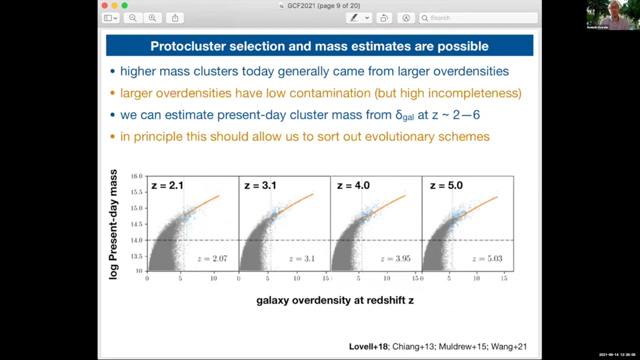 ratchet of about two. okay, lower mass clusters will will typically pass this threshold much later around ratchet one. of course the details between the different semiotic models and the different hydro simulations differ, but in general, i think the they all agree on these, these basic, basic facts, and they also all agree on the fact that actually, it seems that not only the selection 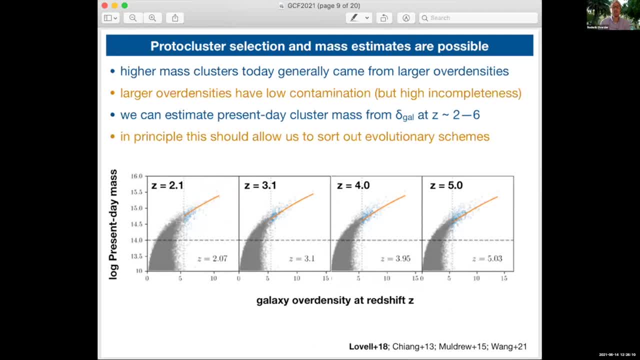 of these systems is possible based on over densities of galaxies or gas in the sky, but all, even estimates of the of the present day masses are are possible. so we know that higher mass clusters today generally came from larger over densities. searching for large over densities of of galaxies or gas selected in some way. 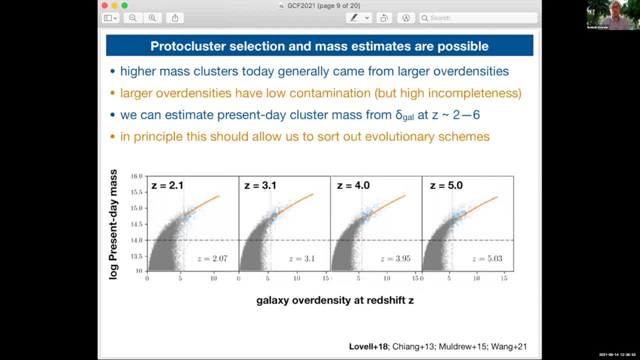 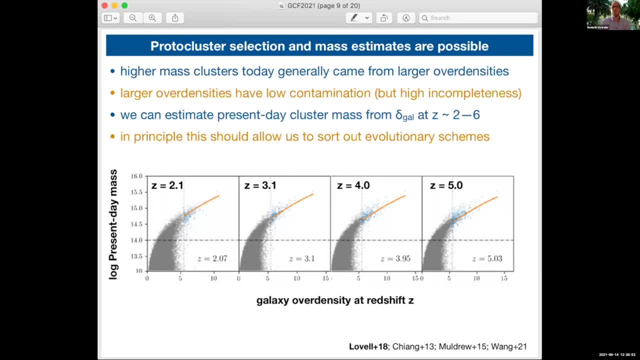 four, five et cetera, actually is is a reasonable proxy of the present day cluster mass within its scatter, and so this means that, in principle, we should be able to sort out evolutionary schemes for clusters and proto-clusters by by by ordering the the objects that we find in these ways. 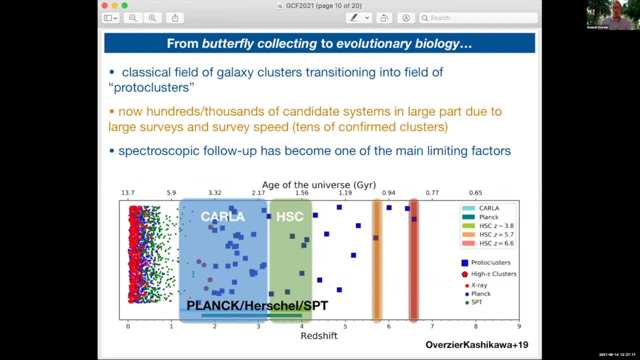 um, so a few. uh, two years ago, we we made this, uh, rather simplistic overview of structures that have been found above redshift ii. i used to call them butterflies, but this figure was also made to actually highlight that that we're that this field is going through a major acceleration. 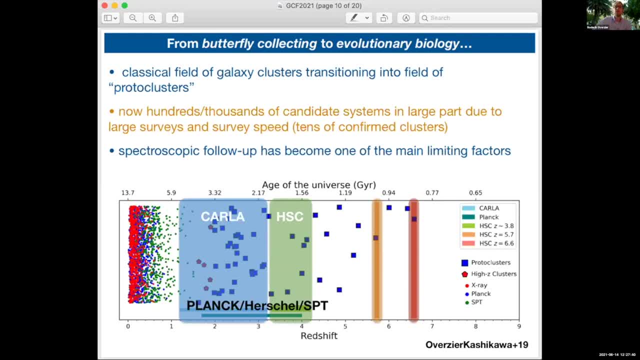 thanks, largely due to large-scale projects, large-scale surveys that are now giving hundreds to thousands of candidates, systems of which, i think many tens have been confirmed as cluster progenitors by now. it also means that spectroscopic follow-up has become one of the main limiting factors. 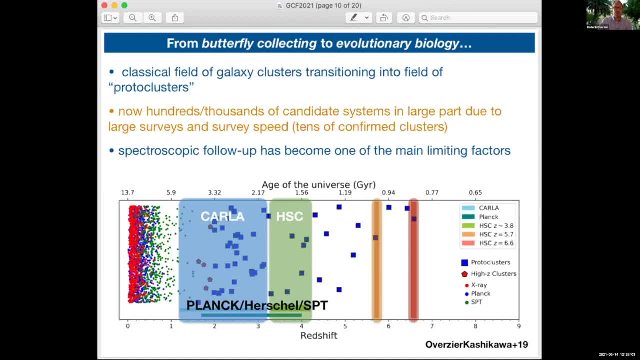 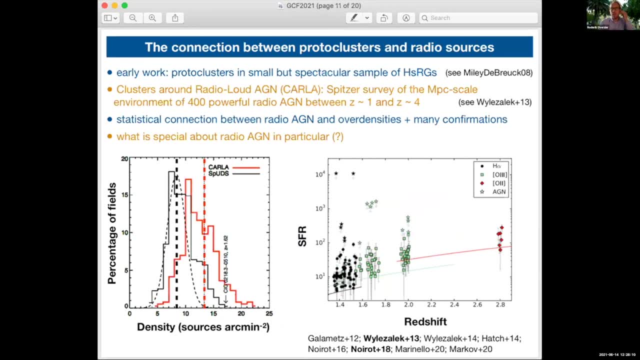 so some of these, these ambitious projects that i'd like to highlight here are the following. so the first project is the carla project. early work showed that proto-clusters appear- uh, appeared in small but rather spectacular samples of high-richard radio galaxies. there's a review. 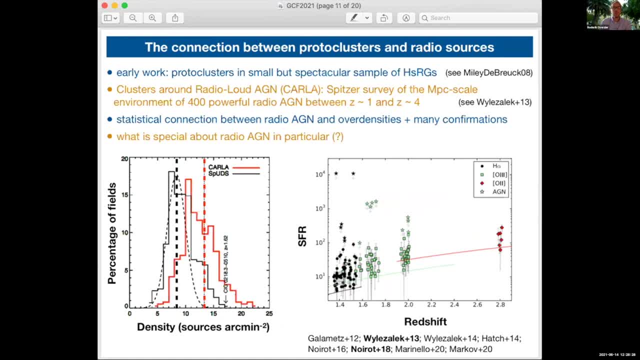 by mighty in the broke 2008 and this was really taken to a next level by the car lab project led by dominica de zalic. at all it was a spitzer survey of 400 powerful radio agn and high redshift and this really showed for the first time the statistical connection between radio agn. 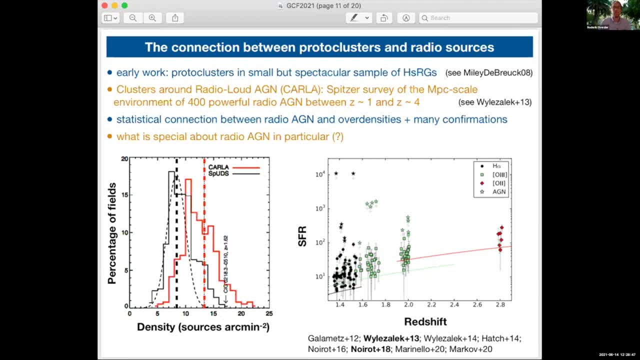 and galaxy over densities and has led to many confirmations since. um, it is still quite not clear to, to me at least, what is so special about the radio, radio agn in particular, that makes them these, uh, these interesting probes of forming clusters, and maybe this is something we can, we can discuss during this, this uh conference. so another game. 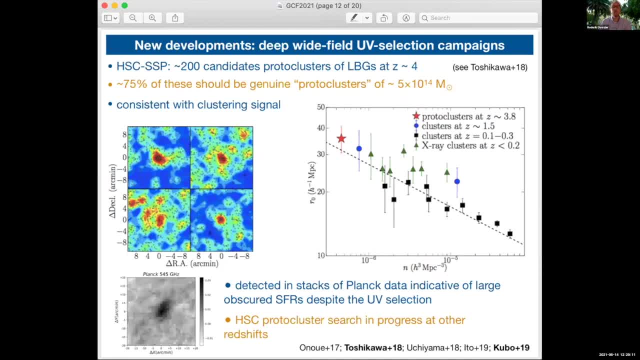 changer, i think, are the wide field deep optical surveys, such as the hyper supreme cam program in the work of toshikawa, and this is a very interesting study. uh, in 2018, uh, a sample was presented of 200 proto clusters for protogluster candidates at redshift4, and about 75 percent of these should be genuine. 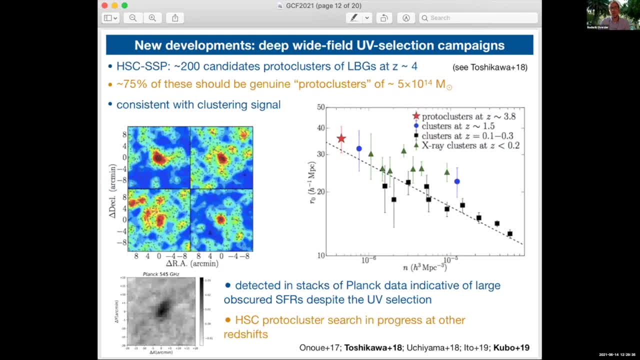 massive objects. they show a clustering signal that confirms this conclusion, and they're also uh detected in a deep stack of plank data, showing that even though these objects are uv selected, they they may harbor uh. also. large obscured star formation rates work with the hyperspring supreme chem imaging surveys being extended to uh to other redshifts. 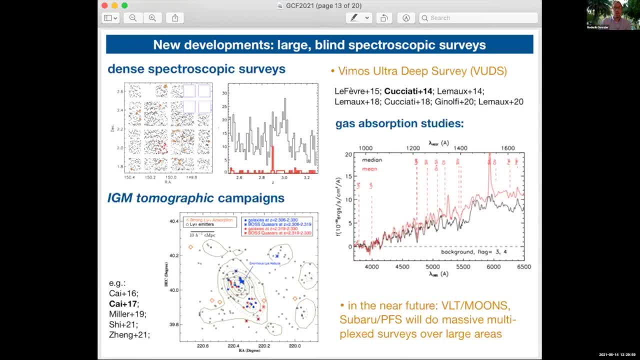 than redshift four. another huge uh surprise, i think in recent years was the the arrival of large blind spectroscopic surveys such as the demos ultra deep survey, these dense spectroscopic surveys. they allow us to find protocols where we didn't know they were or where we weren't particularly looking. the example here of uh over kutcherty. 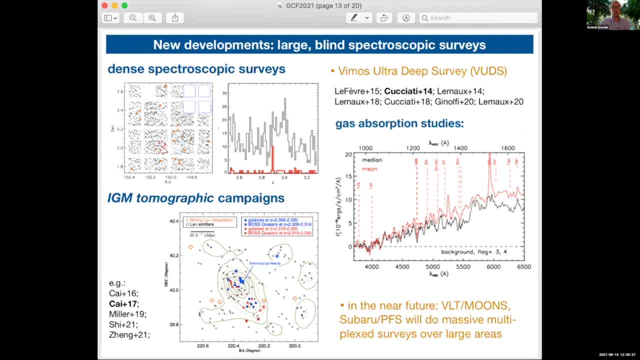 doll 2014 shows you that once you have a redshift of every object you know, in a limited location on the sky, you can pick out the, the dense regions, even when the two-dimensional or the projected distribution of objects on the sky that didn't allow you to to identify these objects once you. 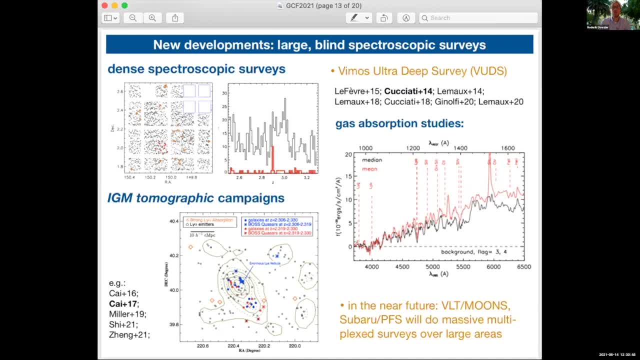 have all these spectra, you can stack them, and this, oh, opens interesting doors to study also the gas components of these systems, such as shown here on the right, And this is related to yet a whole new approach of finding these kinds of systems through tomography of the intergalactic medium. 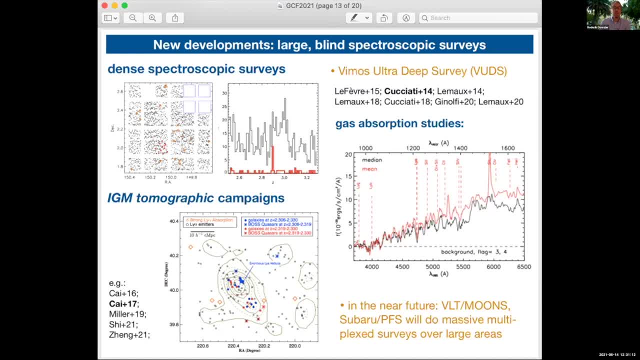 And the example I'll show here from Chiadl 2017 shows a massive structure of galaxies that was purely identified based on the absorption signal that they imprint on the spectra of quasars in the background. In the near future, I think we can expect. 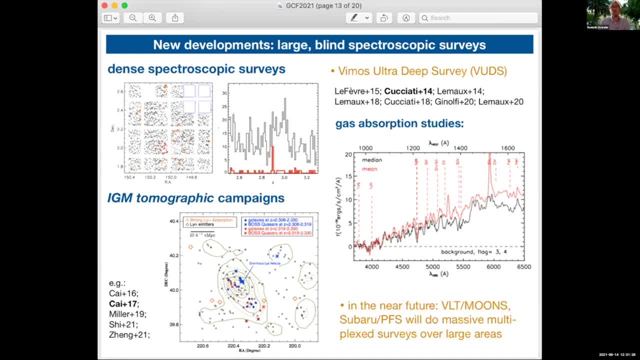 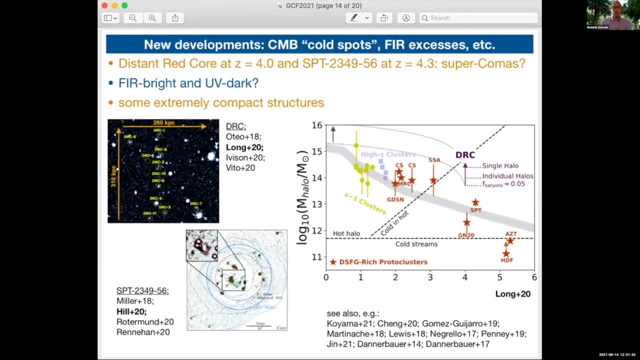 this kind of surveys to really take off with instruments like VLT, MOONS and the Sue-Babel-Prime Trochus Spectrograph that will do massive multiplex surveys over very large sky areas for the first time in history- Another big surprise of recent years, I think. 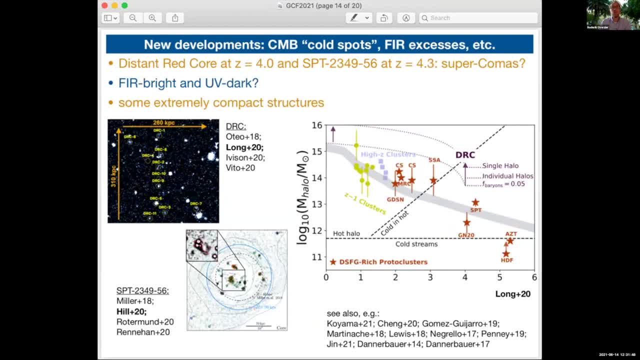 was the discovery of the so-called cold spots in CMB data: excesses of far-infrared submillimeter objects. I highlight two objects that I think we'll hear a lot about this week: the so-called distant red core, Redshift 4. 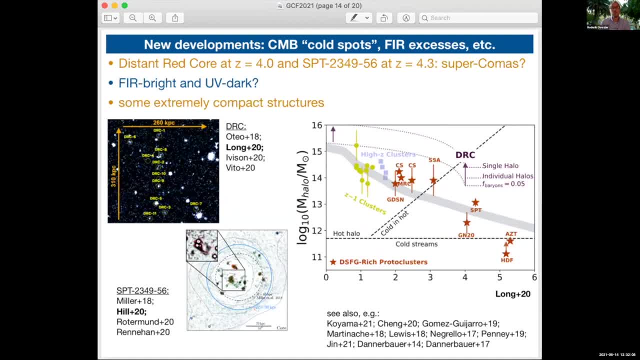 and the SPT2349 super coma progenitors, both at Redshift 4.. They offer also an interesting comparison to the UV-selected systems. It seems we have IR bright and UV dark systems, and perhaps UV bright and IR bright or dark systems. 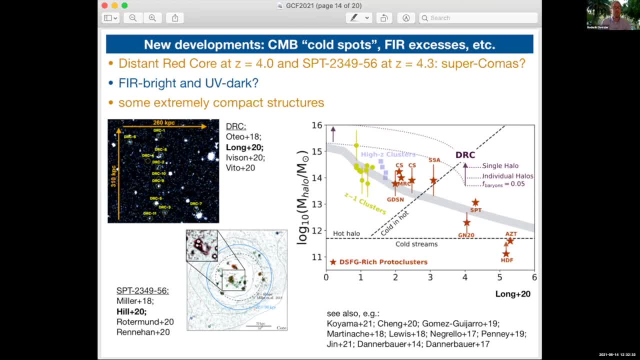 Some of these show extremely compact structures that may signal the formation of a brightest cluster galaxy, And I also appreciate that some of the authors have started to make figures, like here shown on the right from Long Adult 2020, where an initial attempt is being made. 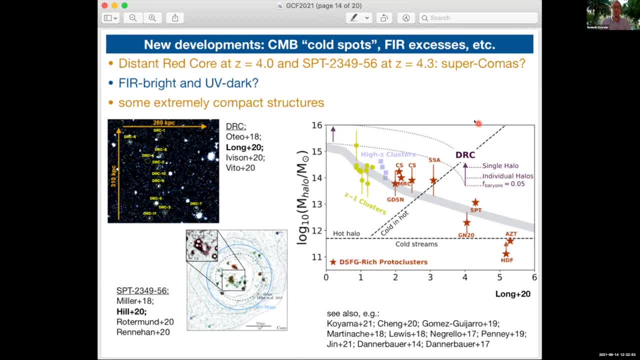 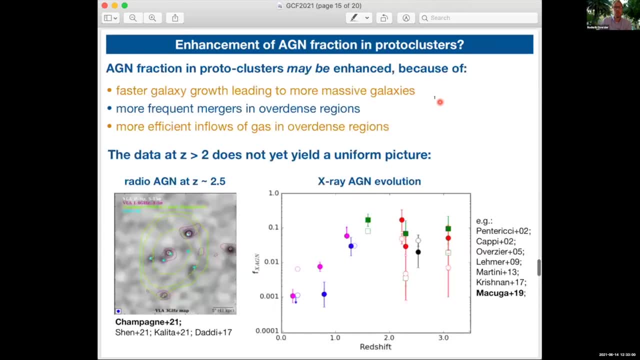 to put the different structures in perspective and compare this to different accretion regimes we may expect, as a function of mass and redshift, Some topics that keep coming back in the study of clusters- project clusters- are topics such as the enhancement of the AGM fraction. 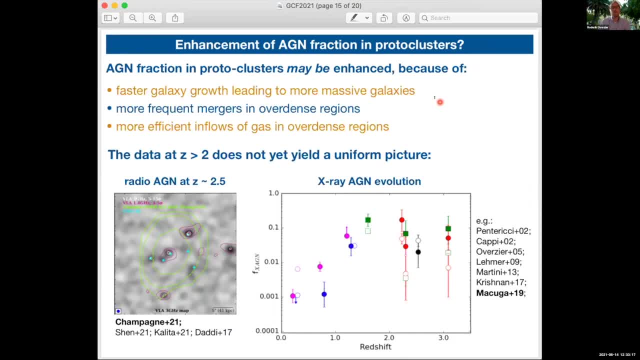 We may expect that AGM are enhanced in proto-clusters, for example, because faster galaxy growth leads to more massive galaxies and more massive galaxies tend to be more frequently active. More frequent mergers may happen in overdense regions or more efficient inflows of gas may trigger AGM. 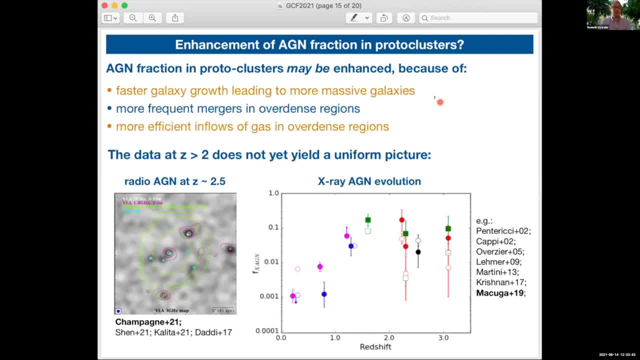 However, the data I think above Redshift 2 does not yield a uniform picture yet. Yes, there are very interesting examples of proto-clusters that harbor many X-ray or radio-selected AGM shown here on the left. figure from Champagne Adult 2021.. 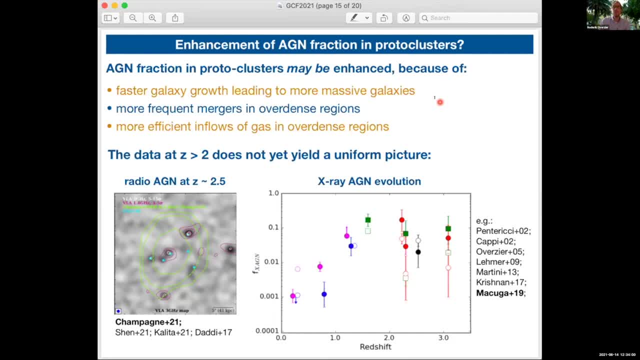 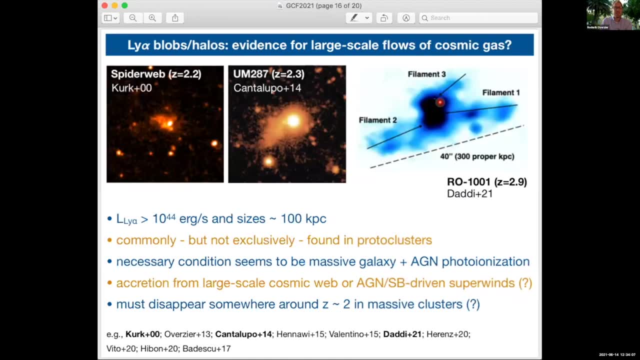 But if you put all the objects together in a plot, I think there's no consistent picture yet. I'm going to speed up a little bit. Another topic that keeps coming back in this cluster-proto-cluster business are the evidence for Lyman-alpha blobs, or halos or filaments. 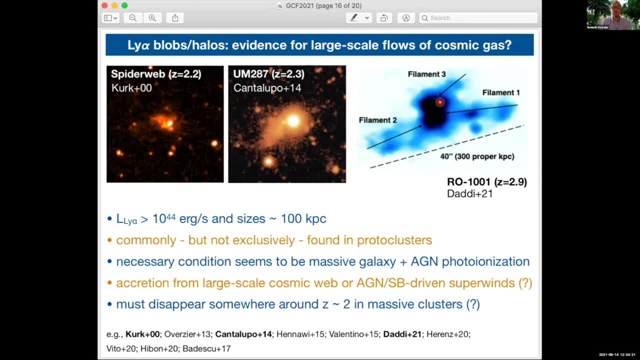 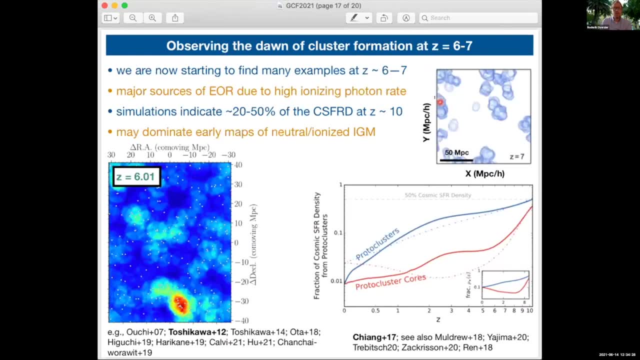 This seems to have some connection to dense environments that we don't quite understand yet, I think, And in the final few minutes I want to take you all the way to the epoch of re-analysation, perhaps, and highlight that we are starting. 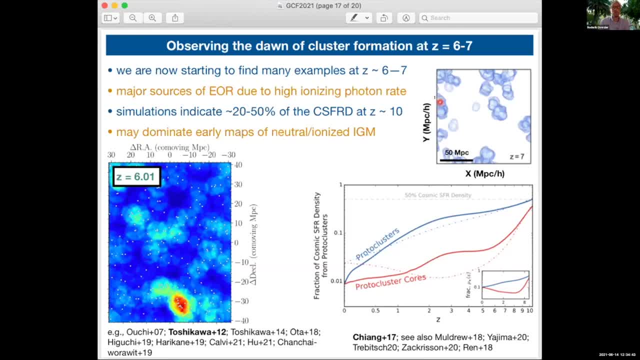 to find many examples of these proto-cluster structures And I think that's a very interesting topic. And I think that's a very interesting topic. We ended up in a喔- multi-lingual cluster systems at redshifts as high as six, seven, eight. 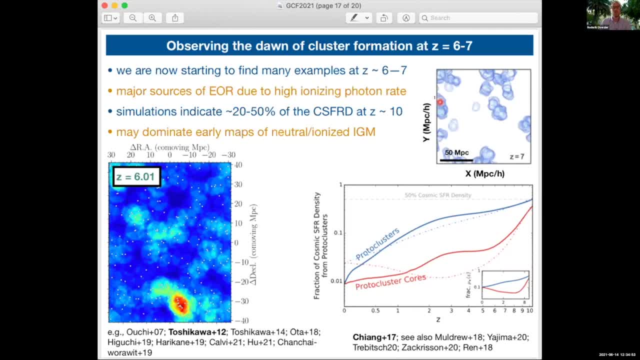 We can perhaps imagine that these would be major sources of the epoch of re-analysation due to their very high ionizing photon rates and large bias. Simulations indicate that several ends of percent of the cosmic star formation rate density could actually be contributed. 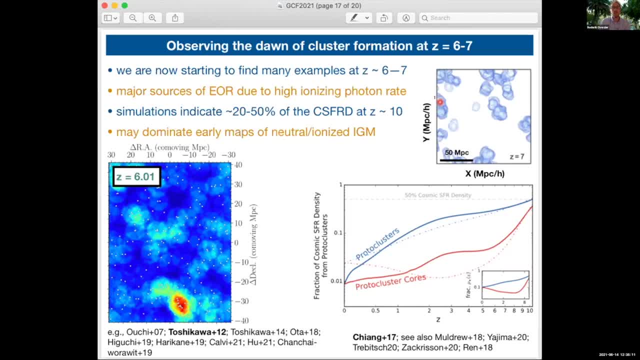 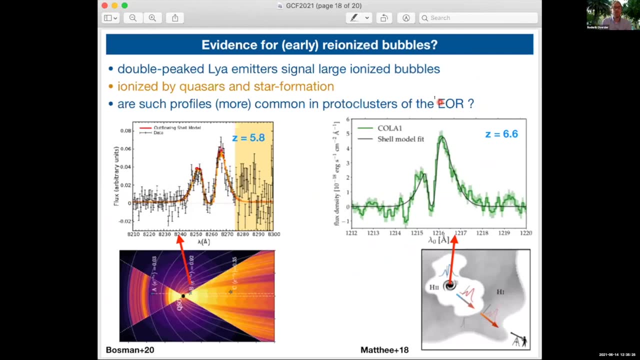 by these large early forming systems, And so they may dominate the midude process a lot. the first maps of the neutral and the ionized IgM that we will be able to make soon. Now here are two examples of interesting Lyman alpha emitters. 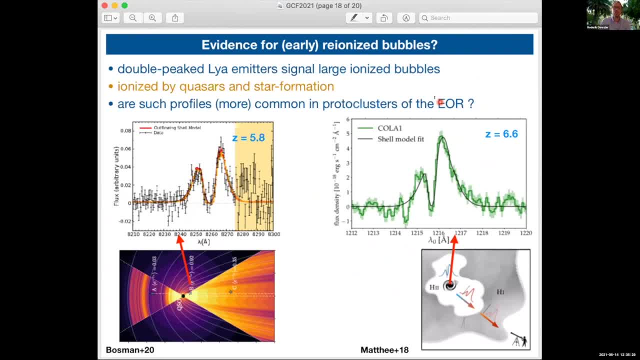 from the EOR- late-stage EOR- that show this double-peaked Lyman alpha emission And this is sort of the smoking gun of objects that are sitting in large ionized bubbles. The example on the left from Bosman, Adult 2020. 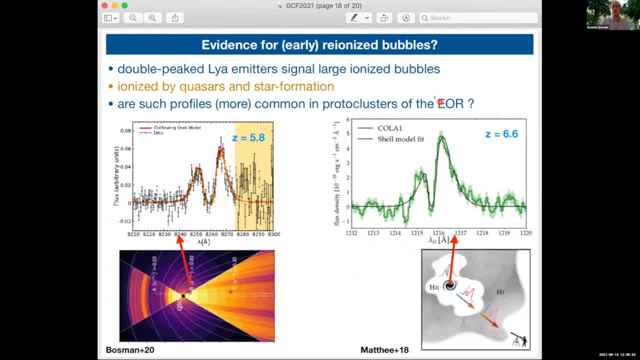 is actually a Lyman alpha emitter that sits in the ionization cone of a quasar at Redshift 6.. The object on the right by Maté et al is a Lyman alpha emitter that probably sits in its own H2-blown large ionized region. 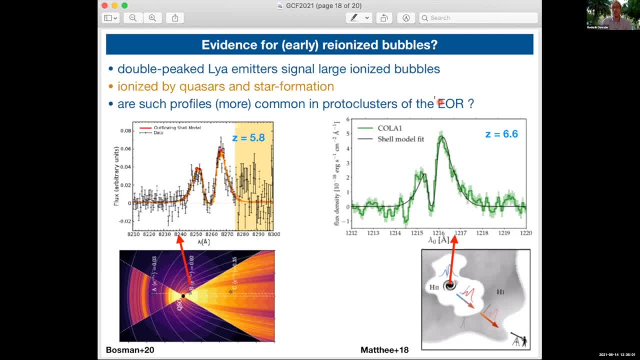 And I think one of the ways in which we might be able to show whether these protoclusters are early re-ionized systems is if we can show that such protoclusters or such profiles like these are common in protoclusters And actually they should be more common in protoclusters. 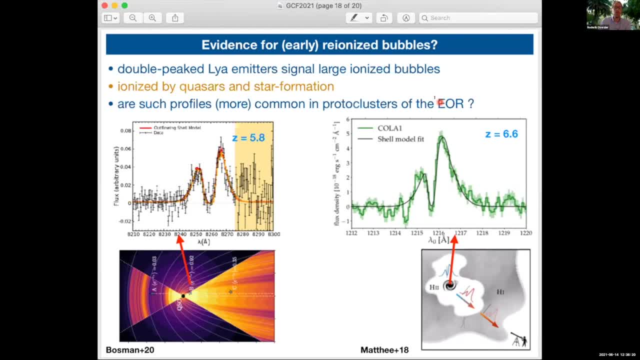 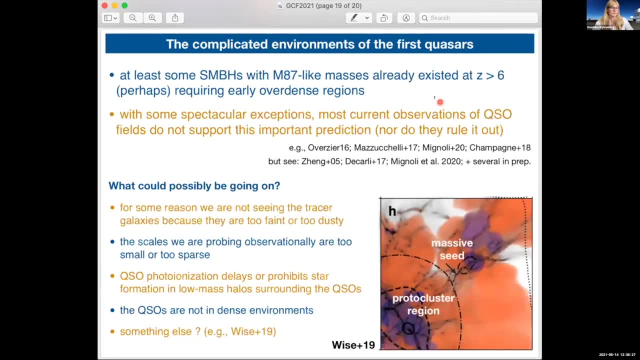 compared to field galaxies at the same Redshift. So I think this will be one way in which we might be able to show this connection between protoclusters and the EOR. My four last slides, Another topic, I think, that will come up today even. 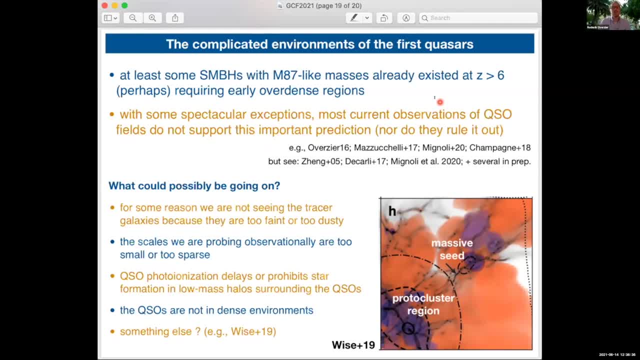 are the complicated environments of the first quasars. I think theory tells us that these quasars- first quasars- should form in the densest environments in the early universe. However, even though some spectacular examples exist, I would say I would still argue. 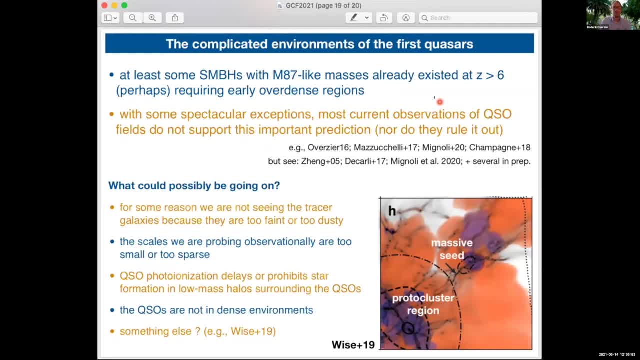 that most current observations of these high Redshift massive quasar systems do not support this important prediction from theory. There's many possibilities that might be going on. Maybe we don't see the tracer galaxies. They are too faint or too dusty. Maybe the scales we're probing are too small. 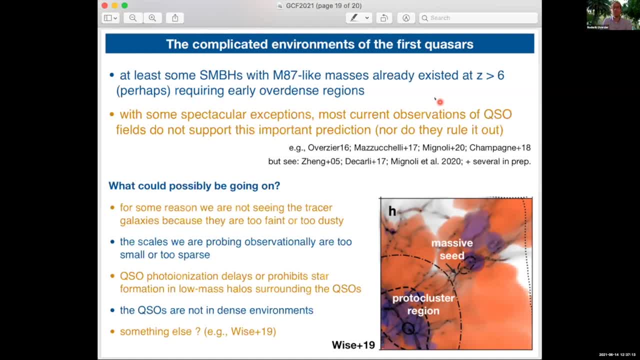 Maybe the quasars are forming in dense regions, but their photoionization delays star formation. Maybe the quasars are not in dense environments, Or maybe it's something completely else, And I invite you to look at this paper by Weiss et al. 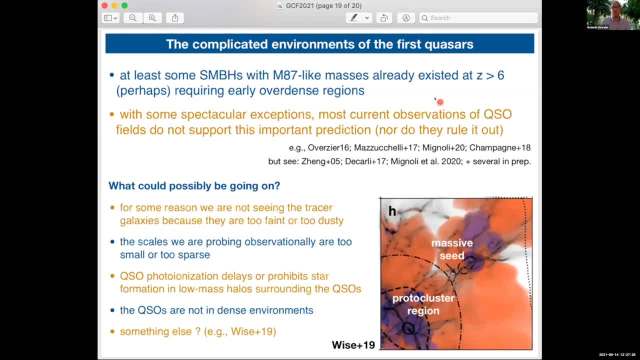 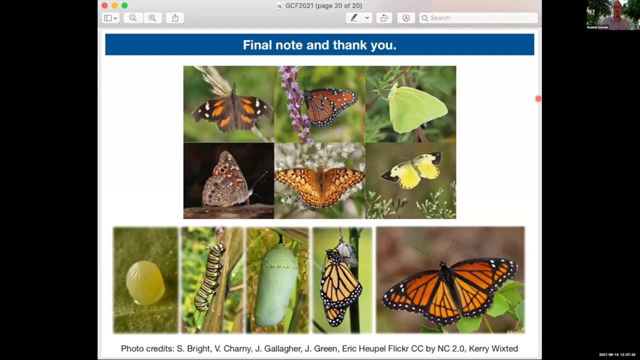 that gives a very interesting idea that maybe the quasars need to form not in protoclusters but near them, because they require a large background UV flux. This is my final slide, Thank you. Thank you very much. In past talks I often have compared the study. 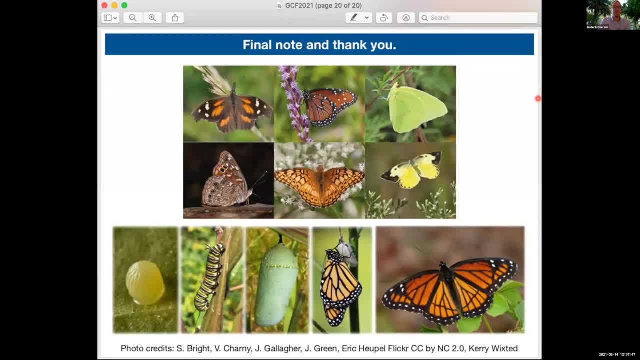 of protoclusters to butterfly collecting. I think we'll see many beautiful butterflies this week and maybe we're finding enough that we can start doing some biology. But actually it's even more complicated, given the many stages in the life of a butterfly. 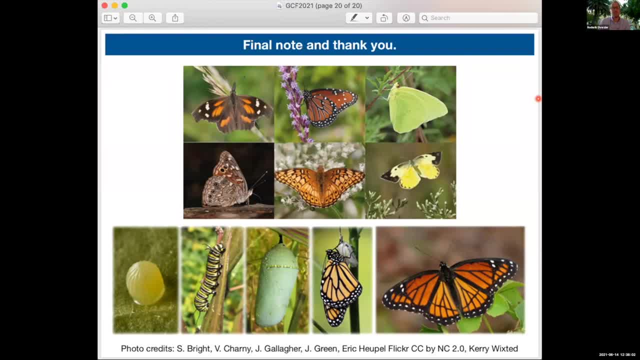 that can look completely different And I'll leave it to you to sort out which stages of the cluster and protocluster are: the egg and the caterpillar and the butterfly. I guess these are the difficulties that we're facing in this field. Thank you very much.